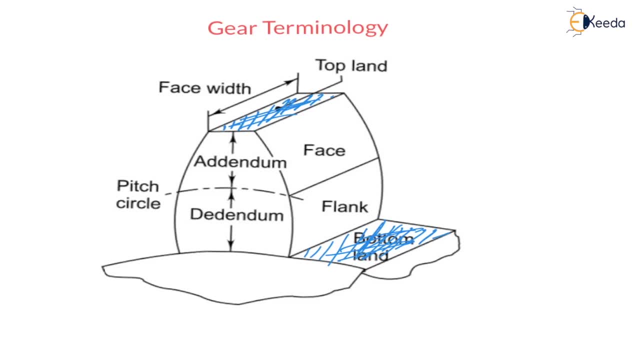 Now again, there will be a pit circle Here. this is very important. There is a pit circle. See, you can find a pit circle. Now, this pit circle is an imaginary circle. We can say pit circle is imaginary circle where pure rolling motion is observed. 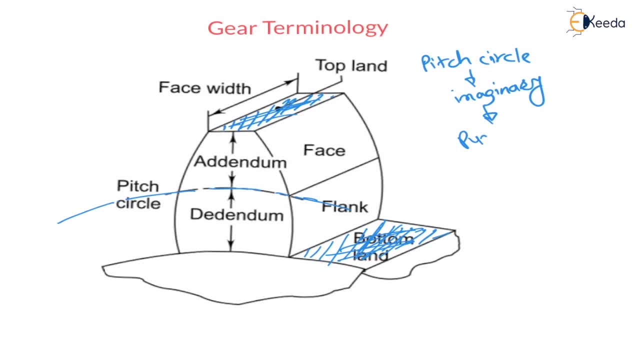 At this pit circle pure rolling motion is observed. Pure rolling motion means only rotation. There is no translation effect. Right At pit circle or imaginary circle, Pure rolling motion is observed, and generally the size of gear is specified by pit circle diameter. 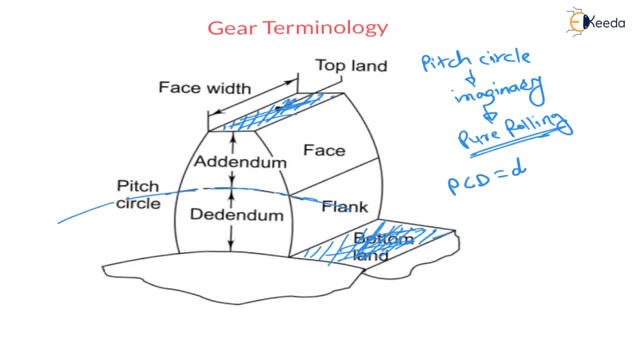 We can say pit circle diameter, which is represented as D, And the size of gear is represented with the help of this pit circle diameter, or imaginary circle diameter. Now, in mating gear. in next diagram we will see again this pit circle for gear as well as pinion. 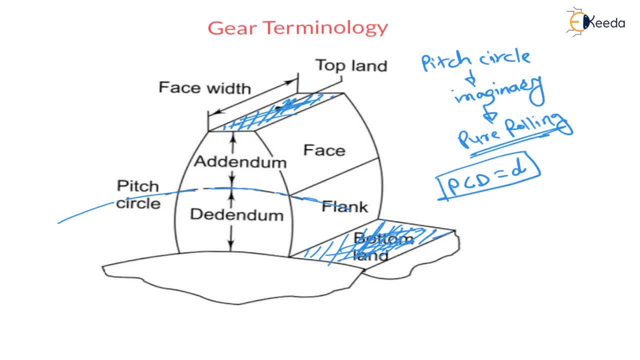 Don't worry about that. Remember, it is an imaginary circle Right Now, at top land. it is called face width. This should be the face width of the gear. Therefore, B is equal to face width. We can say B is a face width. 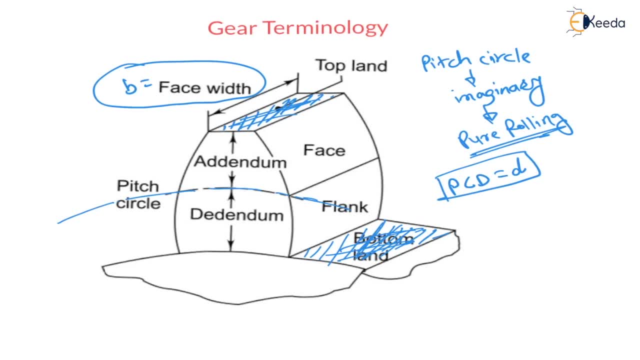 Right Now from pit circle. from pit circle in side view, if I see the upper portion is called face. You can see here this portion is called face, Above pit circle, Right, And the lower portion is called flank. 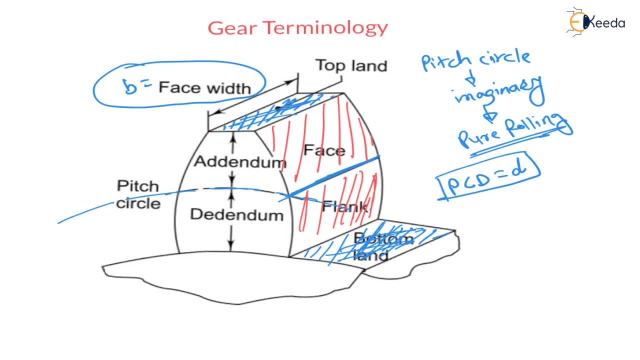 For a tooth. inside view. the lower portion is called flank and upper portion is called face. You can see here the names are given face and flank. Right. You can see here Now from pit circle. the face width or upper portion is at distance. addendum equal to addendum. 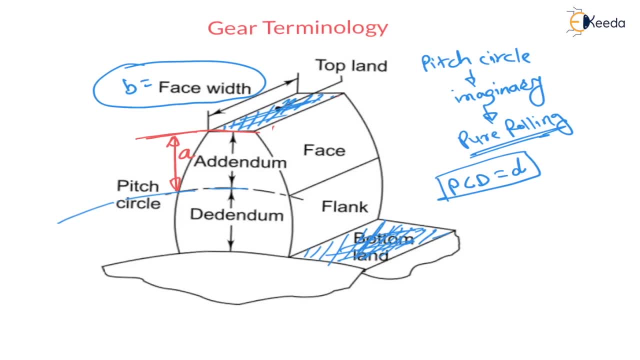 This distance is addendum, we can say represented by A, And from pit circle the bottom or bottom land is at distance, deadendum which is given by A. Therefore we can say here total depth- we can say total depth of any tooth- is nothing but addendum plus deadendum. 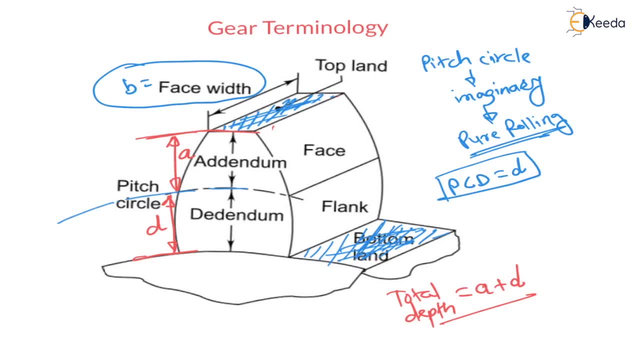 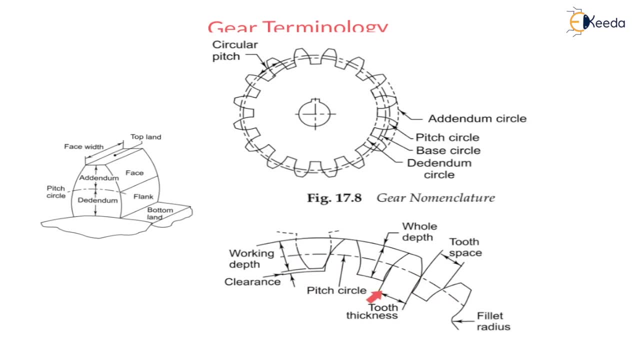 Right, Its addendum plus deadendum is nothing but total depth of any tooth. Now, in full view, this is a gear, total gear, And some parts are given for mating gear. This is the mating portion and this is the gear. 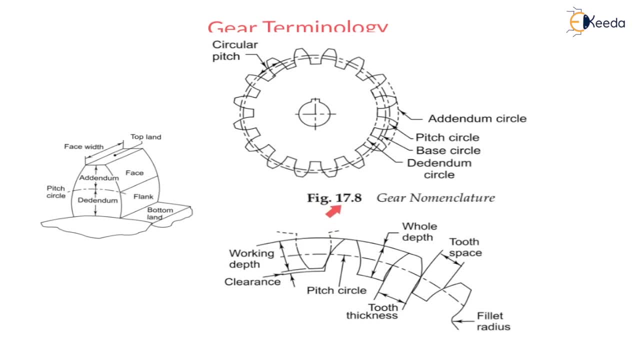 Now I have taken this image from V V Bandari Right. Therefore you will find here figure number 17.8.. Right. Likewise you will see here, because directly I have taken these images from V V Bandari book, which is very good book for machine design. 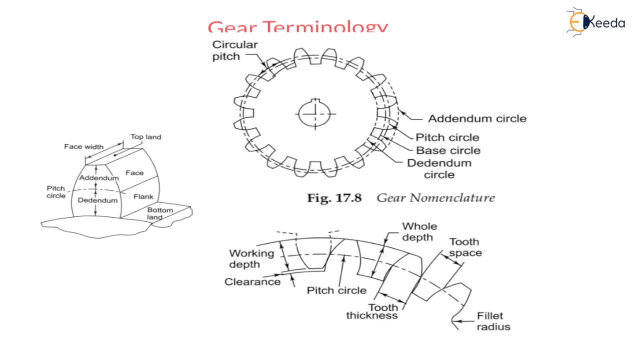 Now this is the center of gear. Right, We can say: let us say center by here. This is the center. Now, from center, if I consider top land and if I draw one circle with the help of center, then this circle is called addendum circle. 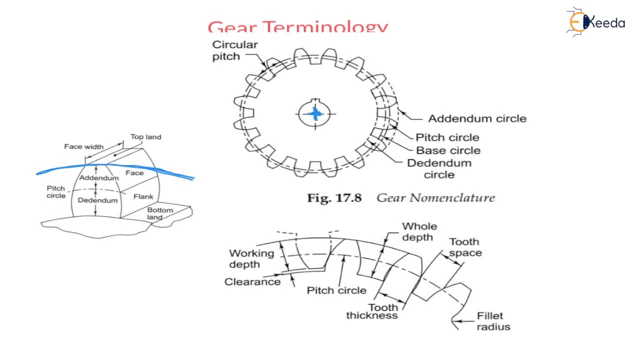 Right, This circle is called addendum circle. In this view, you can clearly imagine, clearly imagine: If I consider all the top lands of all the tooth and if I draw circle, then we will get addendum circle. This circle will be a addendum circle like this, covering all the top lands. 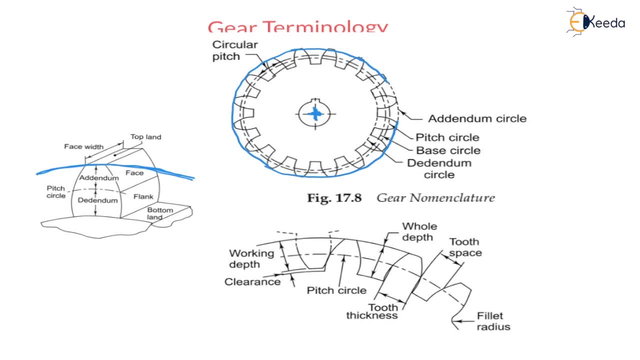 Right. Covering all the top lands, this circle is called addendum circle. Now, and if I cover all the bottom lands here, This circle is called deadendum circle. Therefore, if all the bottom lands are considered to cover the circle, then this circle is called deadendum circle. 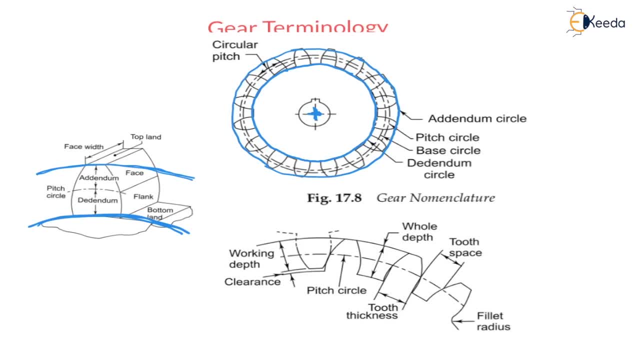 This circle you will see as a deadendum circle. See here it is mentioned. It is a deadendum circle. Right And upper circle is addendum circle. Now let us go for pitch circle. The pitch circle is in between them. 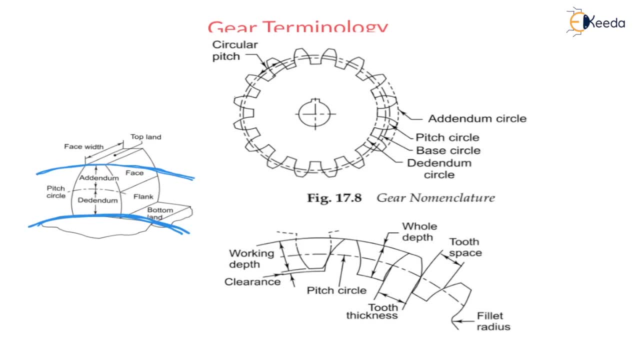 The pitch circle is in between them. See here in the view you can see the pitch circle is here Where the pure rolling motion can be observed. In this diagram you can see the pitch circle. See here there is a pitch circle given. 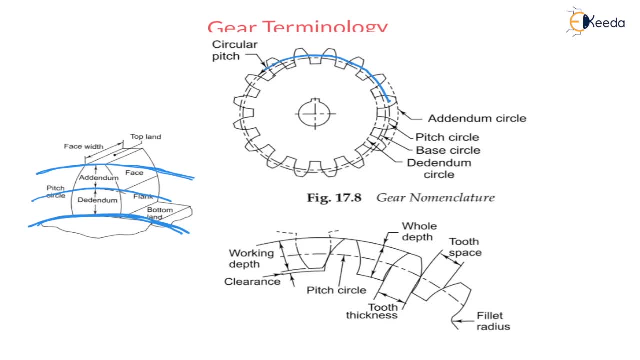 Where there is a pure rolling motion. Right On this pitch circle, there is a pure rolling motion. Below this pitch circle, there is a base circle. What is the significance of base circle? that I will explain. Right. This will be your pitch circle. 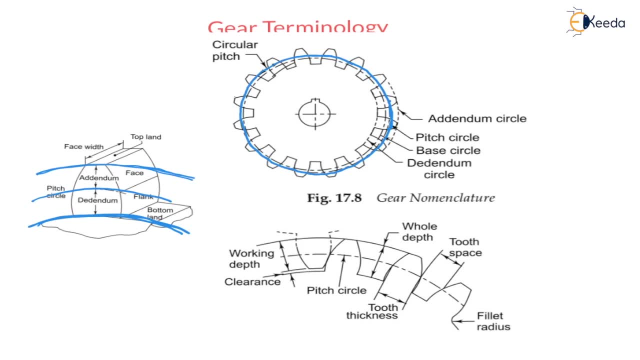 Where, at pitch circle, there is a contact between mating gears. You can see in another view, See here. See, these are the teeths of another gear. These are the teeths of another gear. See, this teeth is for another gear. 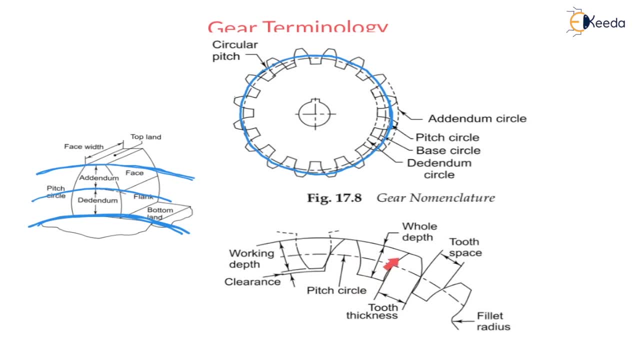 This one And these teeths are on another gear. Let us say, upper side is pinion, lower side is gear. Right Now, these two teeths, This is the- Let us say, This is the teeth of gear 1.. 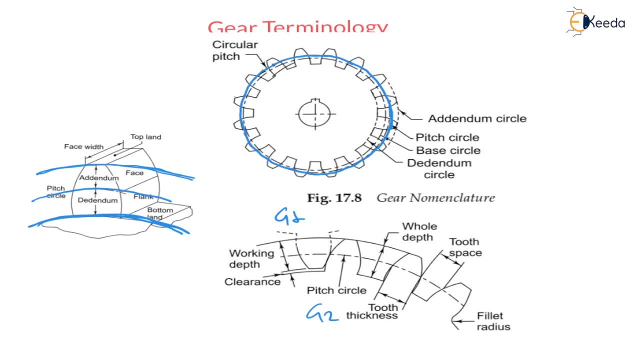 And here it is the teeth of gear 2.. Right Gear 1 teeth And gear 2 teeth. Now they meet at pitch circle, Or at pitch circle there is pure rolling motion between these mating gears. Therefore, here in cross section or in other view, you can see the pitch circle. 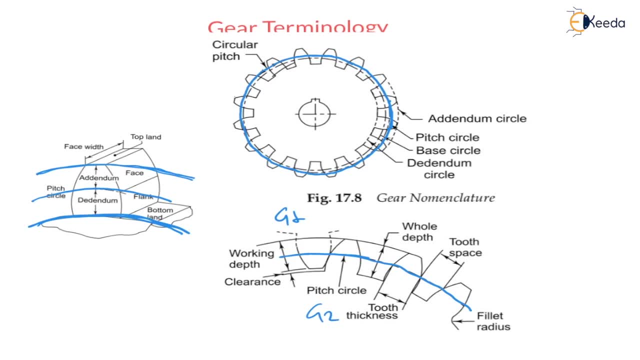 This will be your pitch circle Right, And generally the size of gear is specified with the help of pitch circle, That is, pitch circle diameter. 5D, Which is nothing but pitch circle diameter, is equal to D. Therefore, the size of gear is specified by pitch circle diameter. 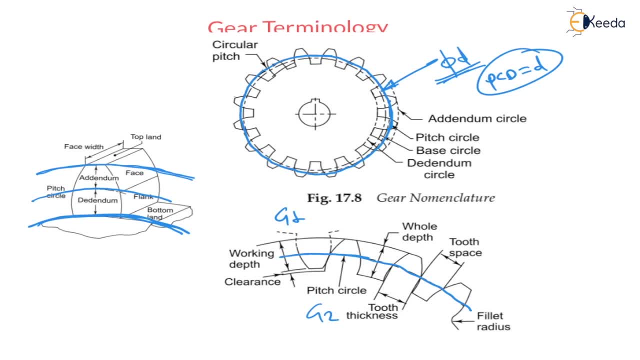 Right Now what we can say Addendum circle. If I want to find addendum circle, this addendum circle will be equal to pitch circle diameter plus 2A, Because both sides, this side, this distance, is A addendum. 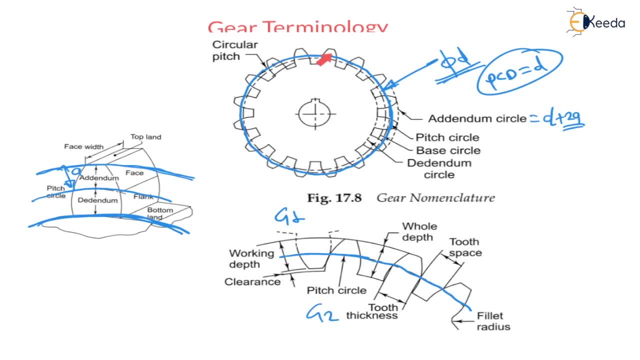 And on another side also. You can see here, This side A upward and this side A downward. That is pitch, circle diameter plus 2 addendum. This we can say: And again there is a dead end of circle. See, dead end of circle is nothing, but this portion is dead end of D. 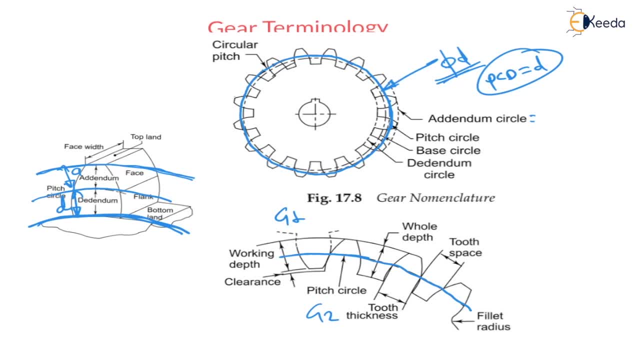 This portion is dead end of D. Here you can see Right. Therefore this side D and this side D. Therefore we have to subtract for dead end of circle From pitch circle diameter. we have to subtract 2D Right. 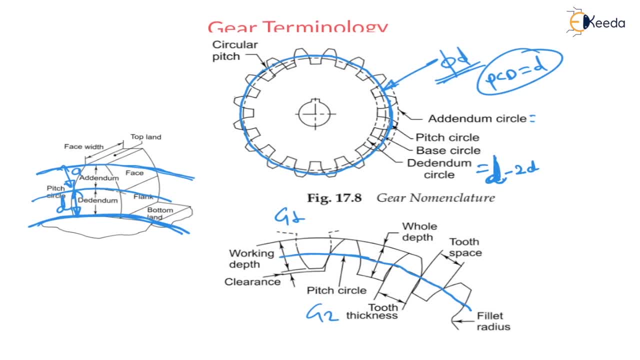 Right, Pitch circle diameter is D And here 2D is dead end of D. This small d is dead end of d. This d is for dead end of d, This d is for pitch circle diameter. Right Again there is one more circle called base circle. 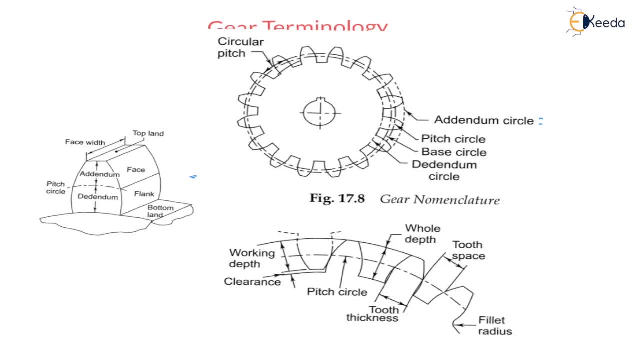 See here, this circle is a base circle. Now see just below pitch circle, you can see just below pitch circle, this circle is called base circle. Now, base circle is nothing, but just below pitch circle there is a base circle. 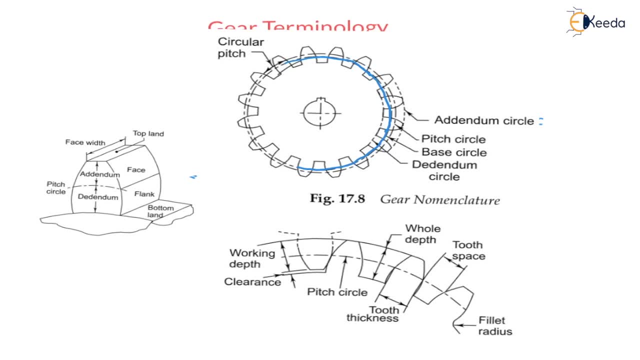 base circle. now, this base circle is not here, but above this base circle this tooth profile is involved. tooth profile is involved. now, this profile we are going to see later. right, let us say there is a base circle like this here below, just below p circle. this is a base circle here. 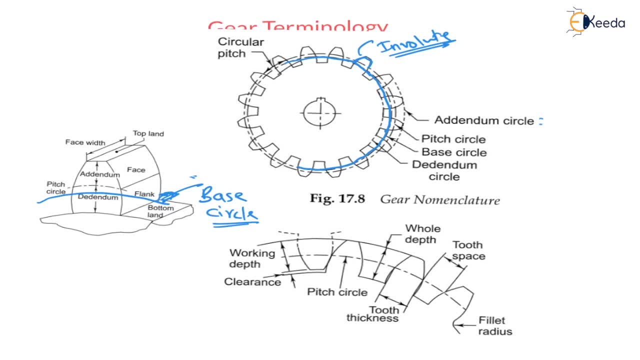 it is a base circle and from this base circle the upper portion is involved. this profile of tooth is involved profile. there is a cyc They portal also that we will see in separately. I will make a video on inavalued and cycler profile. but remember from base circle the upper portion. 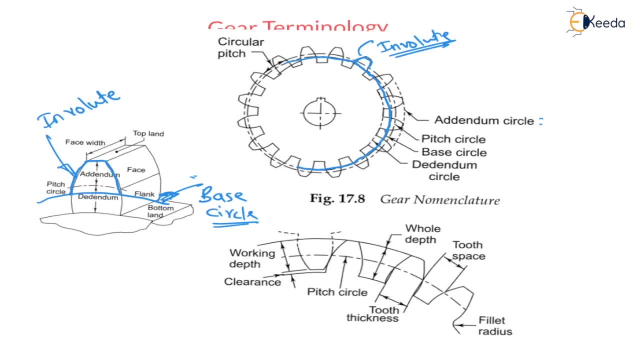 is cut right. that is upper portion is in old. it from base circle. now here you can see two mating gears: this is the 2 of upper gear and this is the tooth of lower gear. now see from this circular P. upper distance is item of 1st gear. 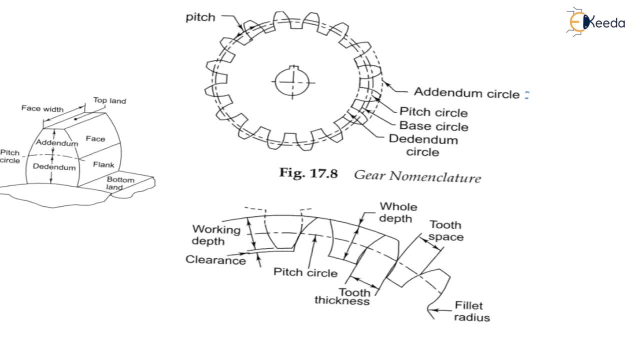 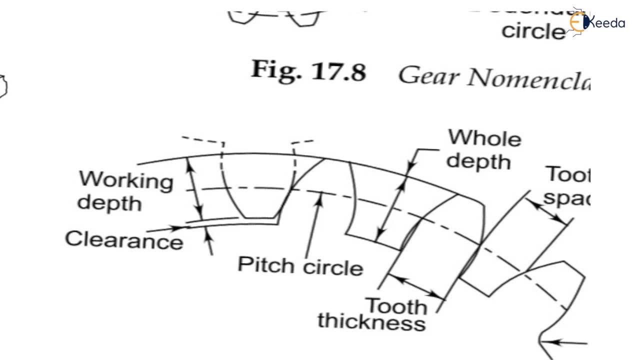 you can visualize here. see, i will zoom it so that you can clearly visualize right for working depth and total depth that we have to see right now. see from this pitch circle- here you will find pitch circle, from this pitch circle the upper portion. this much distance is addendum of first. 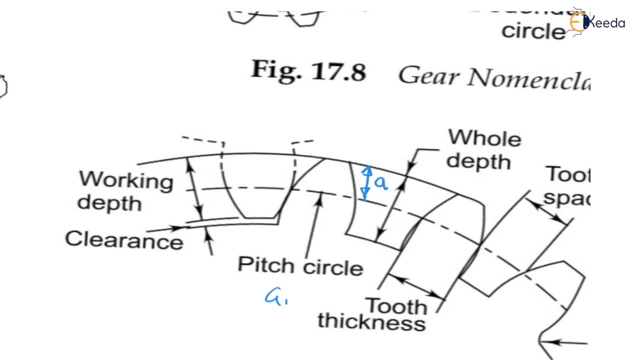 gear. right, that is bottom gear. and from this pitch circle, the bottom portion is again addendum of another gear. let us say gear 2. this is addendum of gear 2 and this is addendum of gear 1. right, therefore, the working depth, this much is a working depth which is nothing but working depth. we can. 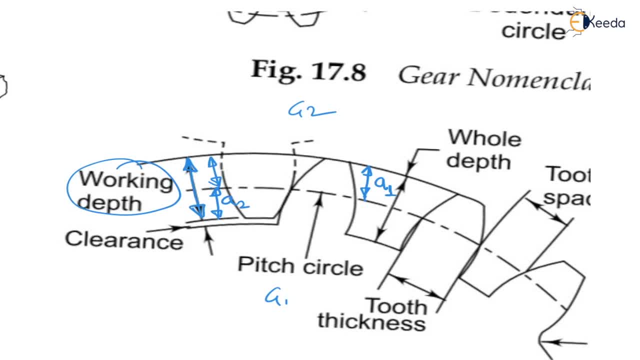 say addendum of first gear. this is the addendum of first gear plus addendum of another gear. means working depth. we can say working depth, which is nothing but summation of addendum of both mating gears. Mating means there is a relative motion between two contacting gears, right? 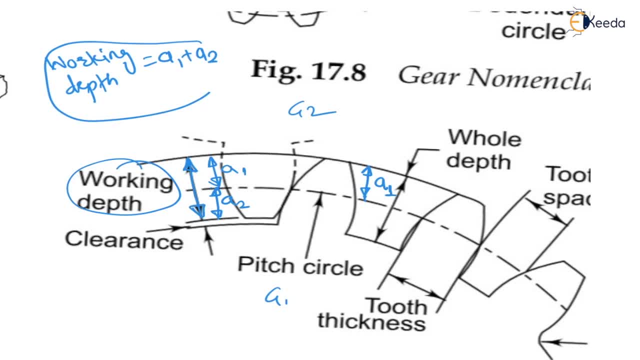 Addendum of first gear plus addendum of second gear, of mating gear. this distance is called working depth. Now you can see again clearance. here you can see clearance. this distance is called clearance. Now this clearance is nothing, but can I say, here it is addendum of another gear. this distance is addendum of second gear. 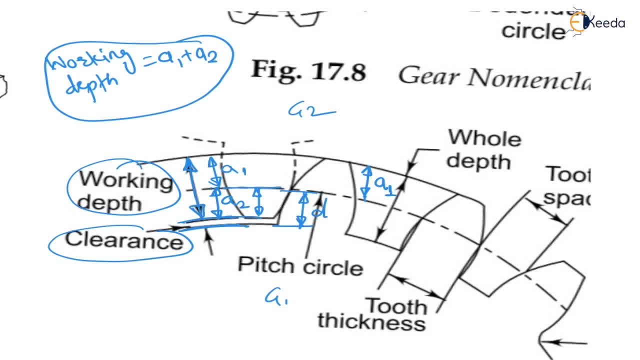 And this distance is addendum of first gear, that is, D1, addendum of first gear. Therefore, clearance is nothing. but we can say clearance is nothing, but this is the difference between addendum of first gear and addendum of second gear, right? 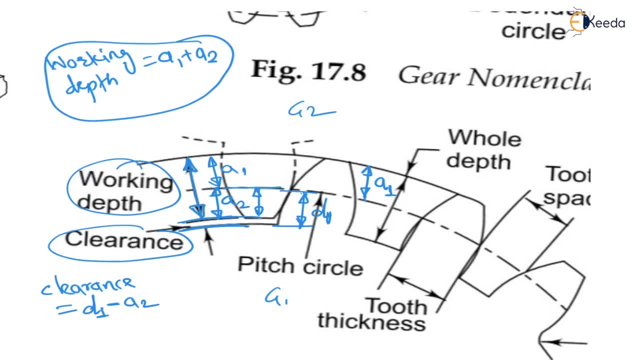 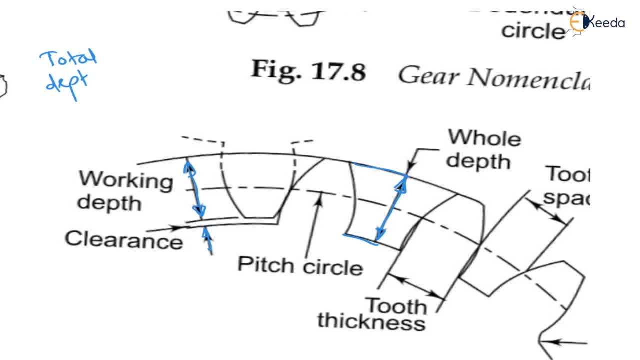 Therefore we can say whole depth or total depth is equal to addendum plus addendum of same gear. My dear students, here you can see this is addendum, this much portion is addendum and bottom portion is addendum, Which is nothing, but we can say working depth. 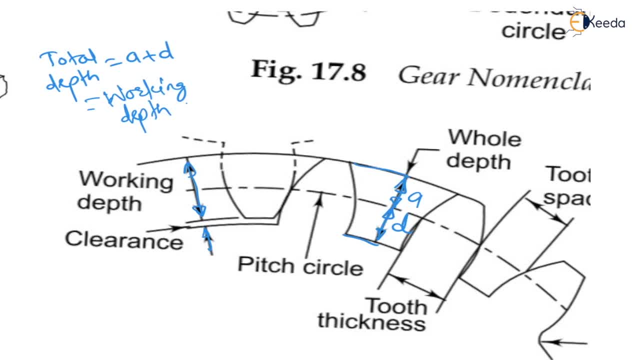 Working depth plus clearance. This is how we can write right. Working depth is nothing but addendum of first plus addendum of second, And clearance is nothing but plus addendum of first minus addendum of second. Then addendum of second will get cancelled. it will become addendum of first plus addendum of first. 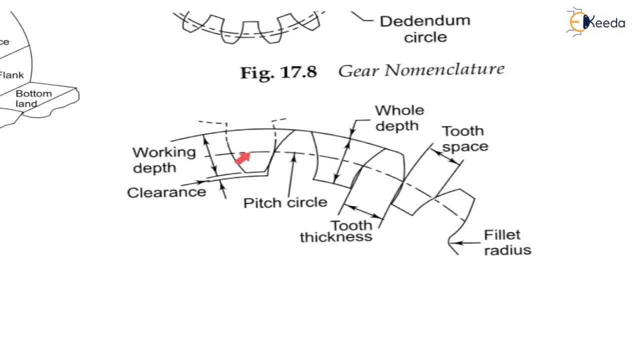 Which is nothing but total depth. Now, at P circle, The thickness of total depth Of tooth is called tooth thickness. You can see here This distance At P circle, This distance is called tooth thickness. right, Therefore, thickness of tooth is considered as at P circle, which is nothing but imaginary circle. 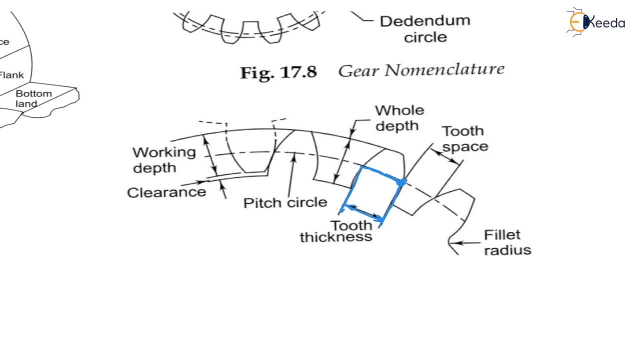 And here the space between this point on the first gear or tooth And another point on the another tooth, nearest tooth. This point is called Another tooth space. Is called tooth space Means In this tooth space The tooth of another gear will enter. 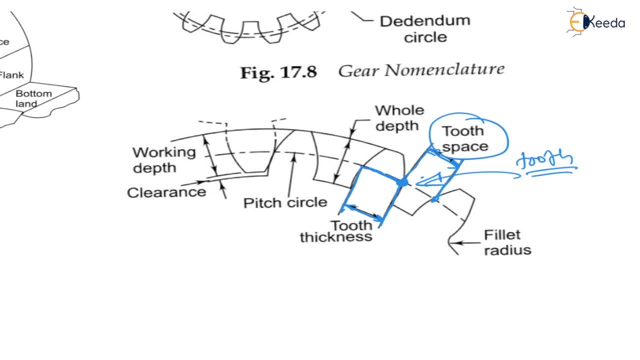 In this tooth space The tooth of another gear will enter. See, You can see in this diagram Right here Means There will be a gear like this. Here there is a gear Or a tooth like this At the tooth space. 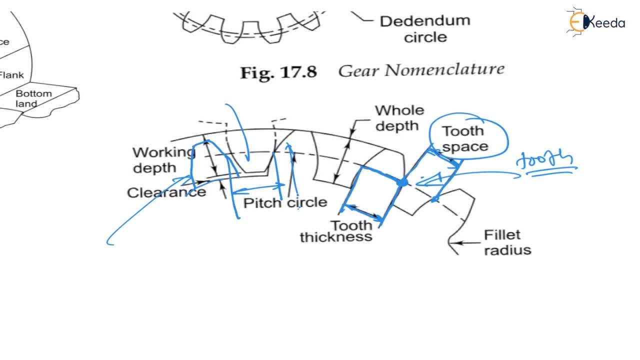 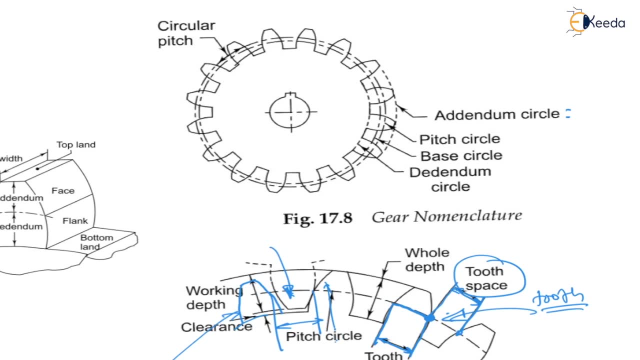 We can say this is a tooth space. At tooth space, Another Tooth of another gear is entering. Now in this diagram. You can clearly see that At P circle This thickness is called tooth thickness. This is a tooth thickness, And 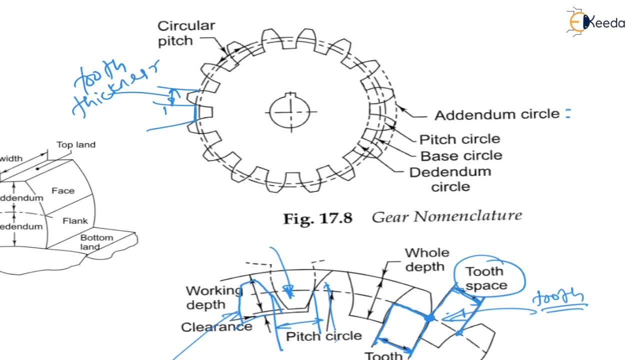 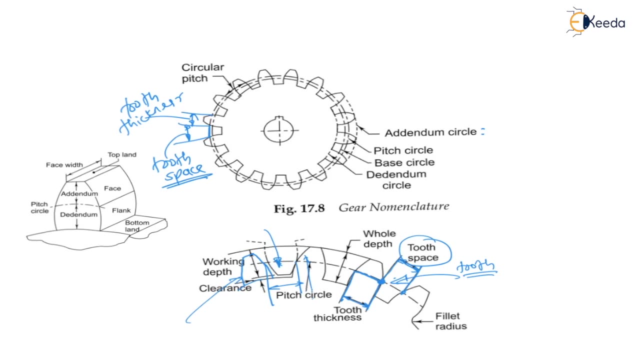 Here, This distance From here, And In tooth space Another tooth of Meeting gear will enter And always This tooth space Is more than tooth thickness. We can say Tooth space is always more than Tooth thickness And it is obvious. 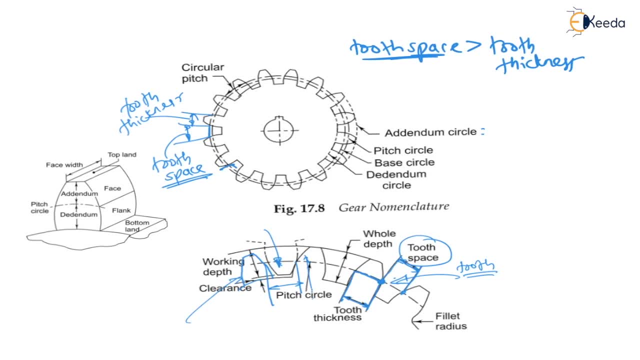 If this tooth space is more than tooth thickness, Then only Another gear tooth will enter into this Space, And this difference is called backlash, Backlash. This difference is called backlash, That is Tooth space Minus Tooth thickness. 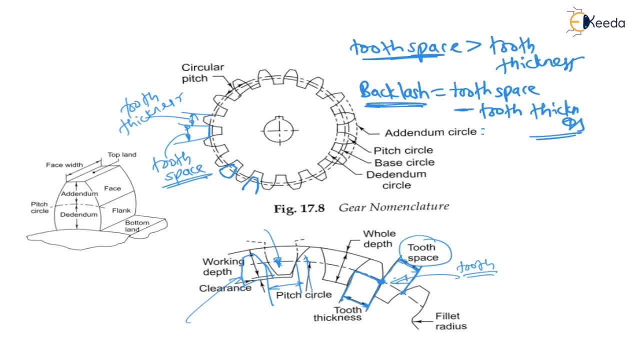 Right. This difference is called backlash, And if backlash is not provided, Then The tooth of another gear will not enter into this Right And The tooth of another gear. Therefore, To avoid jamming between two gears, Backlash is always provided. 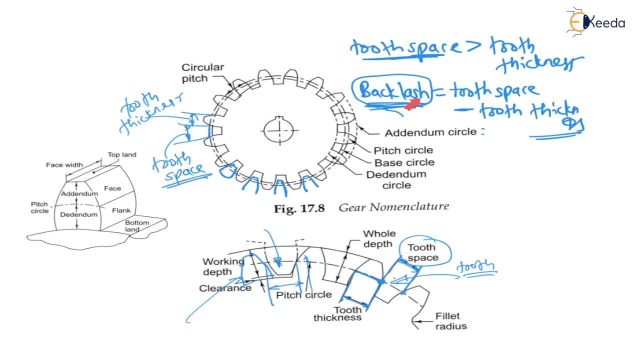 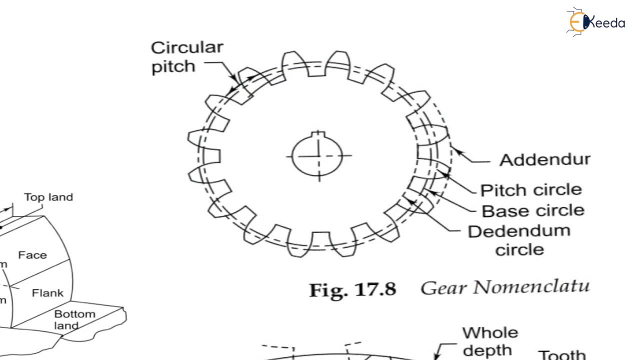 One more reason to provide this backlash is To prevent jamming of tooth. Due to thermal expansion Because of heat, There are chances of increasing the thickness of tooth. Therefore, If, because of temperature, Thickness increases, There may be a jamming. 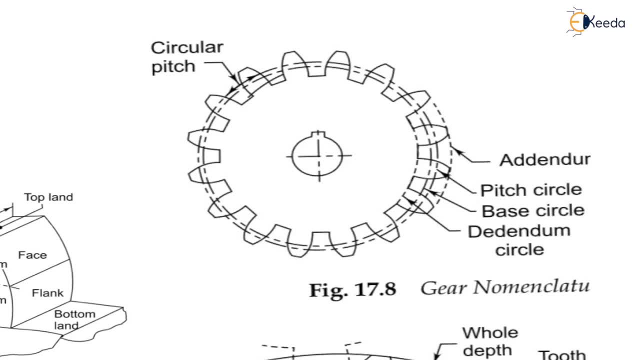 So to avoid this Backlash is always provided. Now, circular pitch is nothing But distance between Circular, distance between two conjugative Tooth, That is. Let us consider, If I consider this point At pitch circle, If I consider this point on the 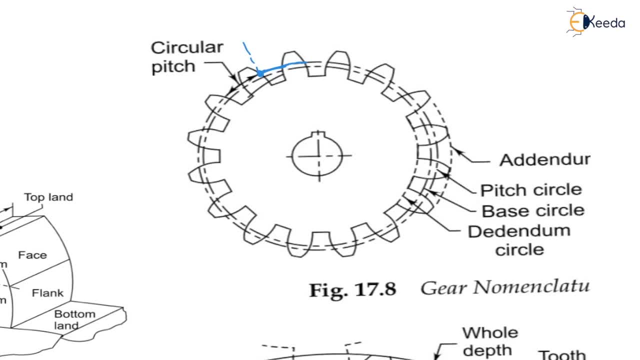 Tooth, Then on the nearest tooth I have to consider same point in circular way, At pitch circle, This point, Circular pitch. Now you can imagine here, In circular pitch, From here to here, There is only one tooth. If I go for another circular pitch, 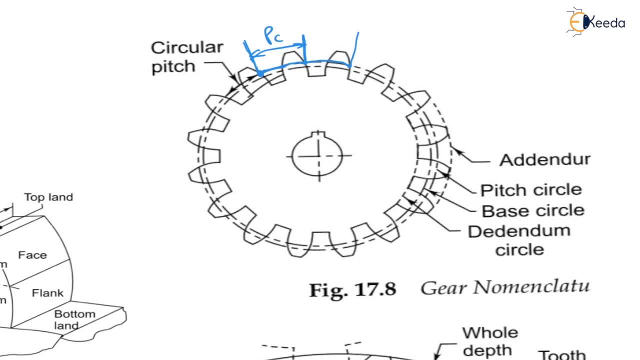 Let us say, From this point to same point on the nearest tooth, This distance is another circular pitch PC. Now see again Between two PC From here to here, This I can say it is a two PC. This total distance is two PC. 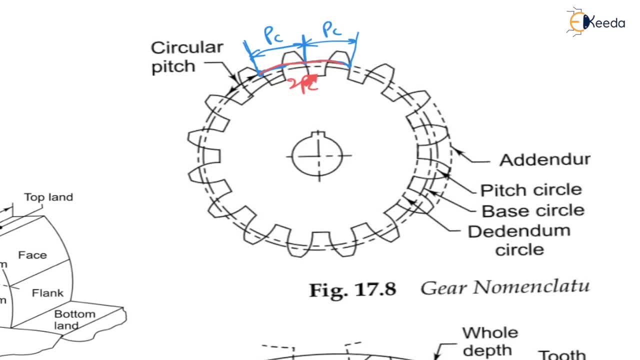 In circular pitch There are two Tooth. This is tooth number one. Tooth number two Means: Let us say There are Total number of tooth. are T Total number of teeth? Total number of teeth Are equal to T. 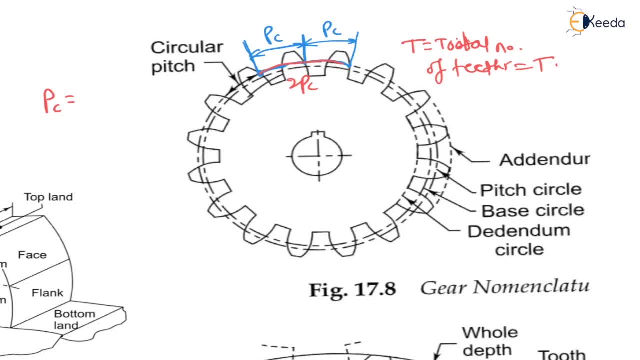 Now this circular pitch. We can say: this circular pitch Is nothing but One circle, is nothing but Pi into D, That is pitch circle diameter, Pi into pitch circle diameter Divided by number of teeth. Because in one pitch circle 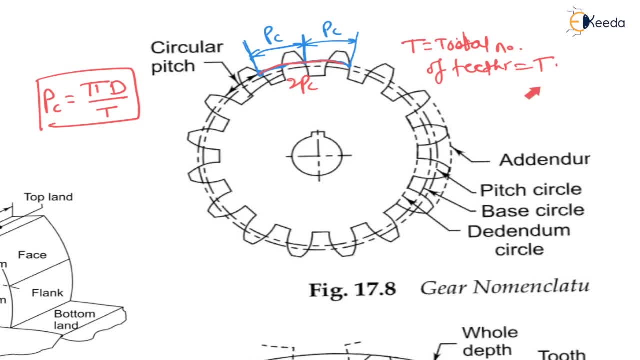 There is only one teeth Right. Therefore we know how many number of teeth are on this gear. Then this circular pitch is equal to Pi D, which is nothing but Circumference divided by number of teeth Is number of teeth. Hence, simply, we can define as: 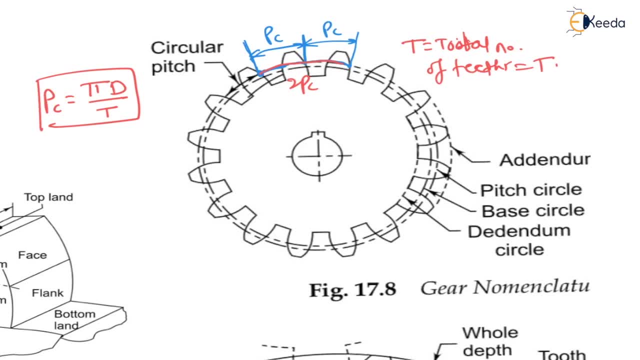 Circular pitch is Divided on adjacent teeth Between two similar points, See Here. this is one point And the similar point is here. This distance is circular pitch, See, we can consider any other point also. Let us consider this point. 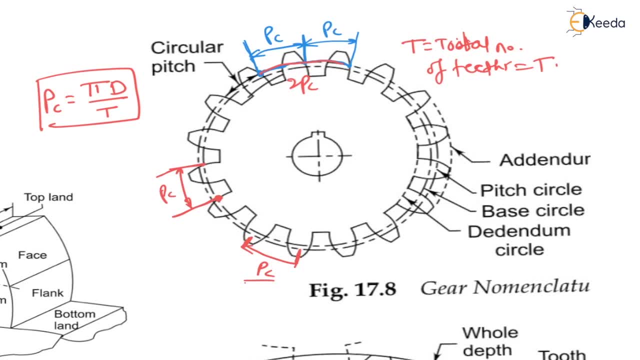 The same point we have to consider. This is circular pitch. Right Here half tooth and here half tooth Means in one circular pitch There is only one tooth. It is equal to Pi D divided by T, Where D is pitch circle diameter. 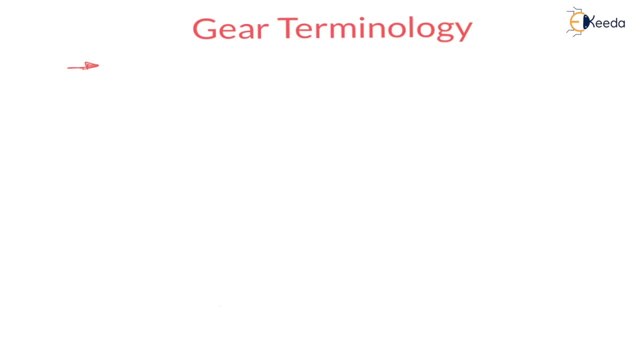 Now, very important point Regarding circular pitch is that For two mating gears Circular pitch must be same Right For two mating gears. Mating gears means the gears Having relative motion between them. Mating gears, Pc must be same. 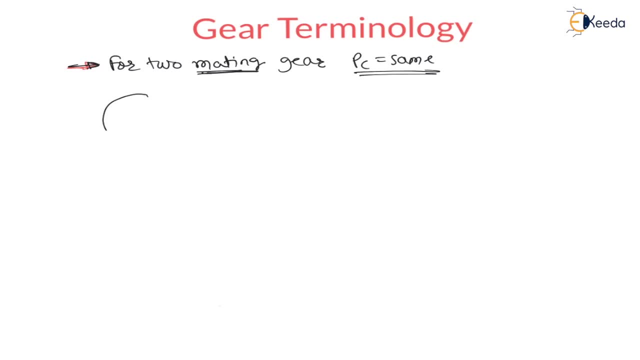 Circular pitch must be same. Therefore, Let us say: this is a smaller one, Pinion Right, And there is a gear Here. I am drawing pitch circles To represent gears. We are using pitch circle Here. it is a pitch circle. 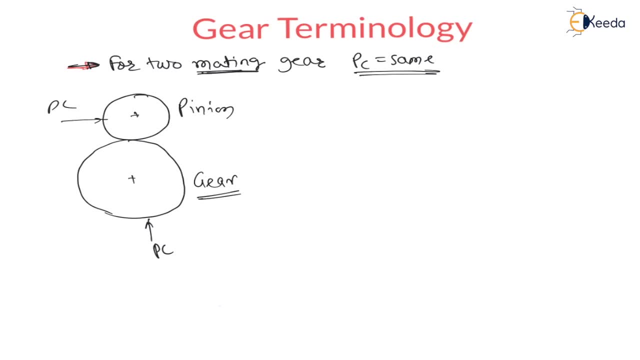 Here it is also pitch circle of pinion. Right Now, for this pinion, Let us say radius is R1.. And for this gear, Let us say radius is R2.. Right Diameter of pinion, Which is equal to diameter of pinion. 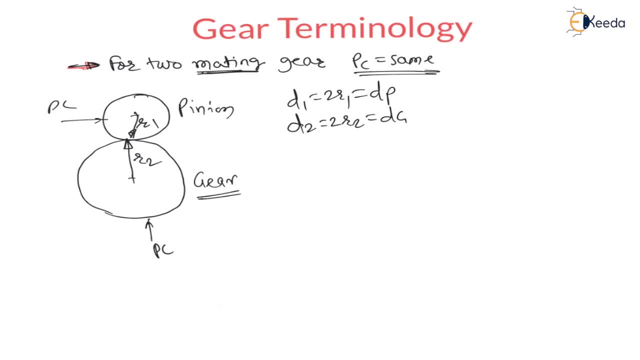 And D2 is equal to twice R2.. Which is equal to diameter of gear Right And circular pitch. Pc1 must be equal to Pc2.. That is Pi Dp. You have a number of teeth on pinion Tp. 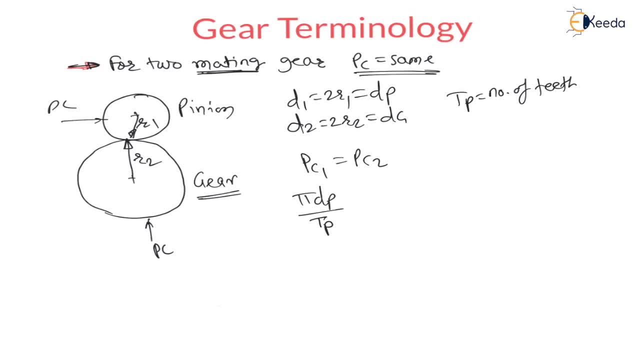 Tp is number of teeth Or tooth On pinion Right Is equal to Pi, Dg. You have a Tg. Tg is nothing but Number of teeth On gear Right And Dg is pitch circle diameter of gear. 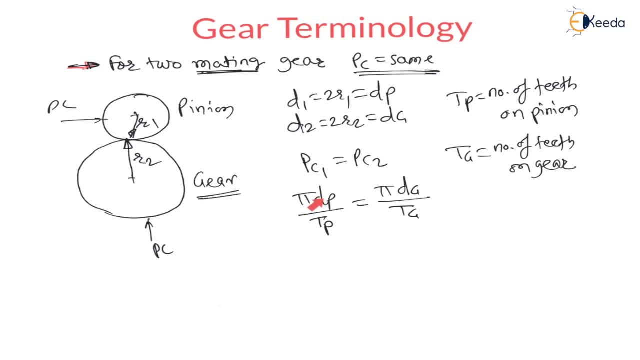 And Dp is pitch circle. diameter of pinion. That we can understand. Right From this We can say: diameter of pinion, Number of teeth on pinion, Is equal to diameter of gear, Number of teeth on gear Or diameter of pinion. 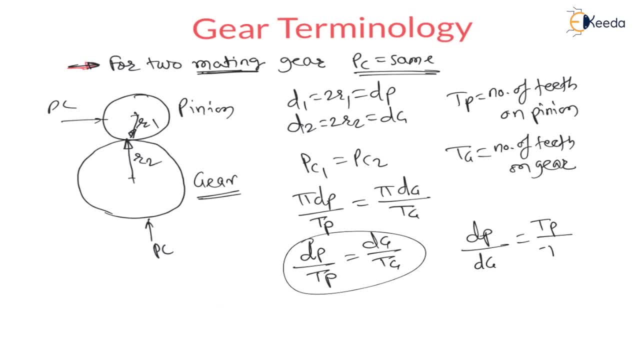 Is equal to teeth on pinion Developed by teeth on gear. That means Diameter is directly proportional to teeth, Means The gear having larger size Will be having more threads Or more teeth. It is obvious Gear having more diameter. 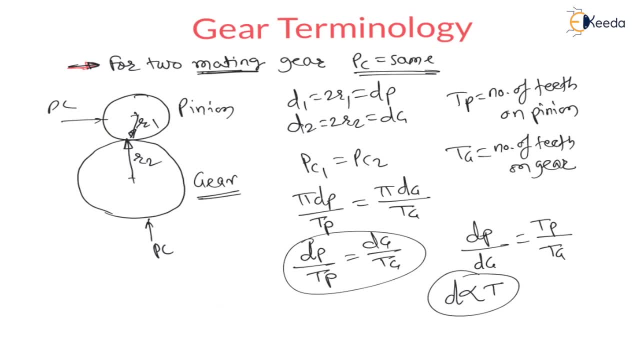 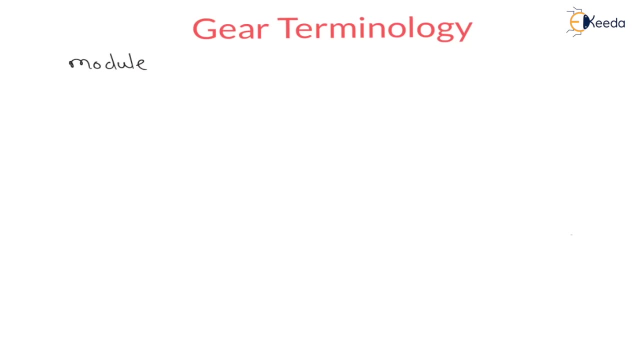 Will be having more teeth And the gear having lesser diameter Will be having lesser teeth. Right. Therefore, on gear There are more number of teeth As compared to on pinion. Next definition is module, Which is also very important Parameter in gear. 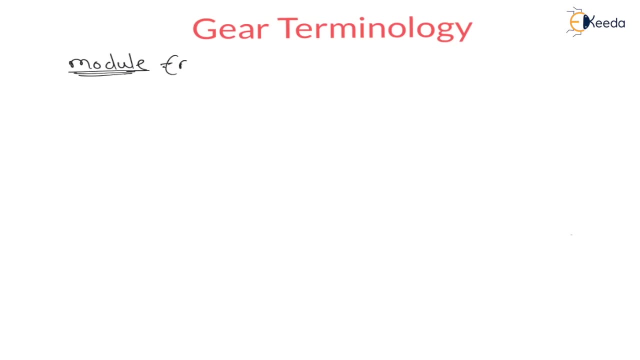 Because many times module is very, very important. Module is nothing, but represented by M. It is nothing but It is a ratio of Pitch circle diameter to number of teeth. Right Pitch circle diameter to number of teeth, That is, Pitch circle diameter to number of teeth. 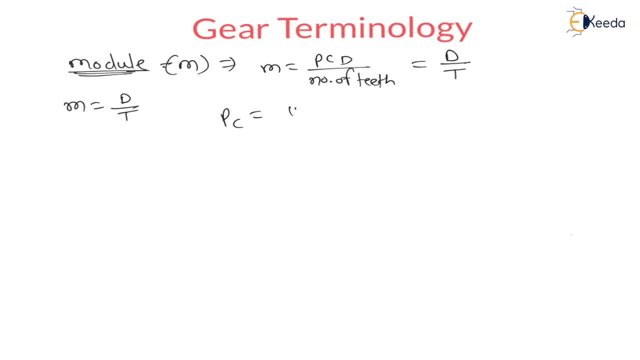 Pitch, circle diameter to number of teeth And circular pitch is Pi D divided by T, Which is pi times M. Therefore, circular pitch is pi M. Right, This is very important, My dear students, But this module is not dimension, It is not length. 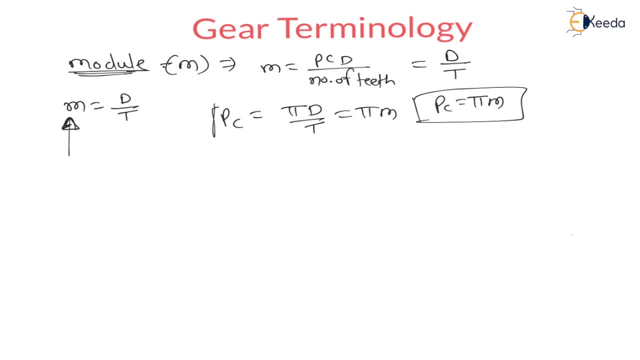 Pitch circle is length But module is not length And generally the gears having same module Met each other Right And circular pitch. Then there is same module Because pi is constant. We have seen formatting gears: PC1 is equal to PC2.. 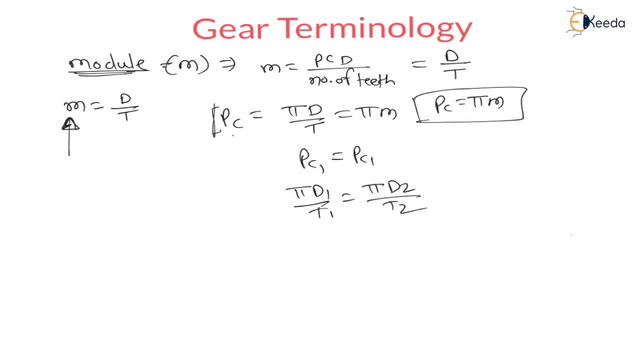 Which is nothing but pi D1 divided by T1.. Is equal to pi D2 divided by T2.. We can say Therefore: pi M1 is equal to pi M2.. Pi pi will get cancelled. Therefore, formatting gears Module is same or constant. 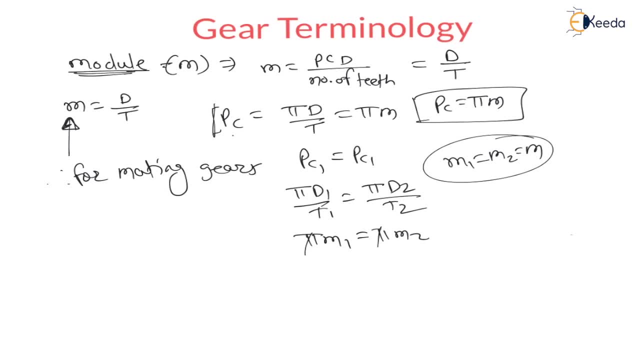 Therefore we can say: For mating gear, Module must be same. This is must condition. Now, next definition is Diametric pitch. Diametric pitch, Now diametric pitch is Represented by PD And this diametric pitch is a reciprocal of module. 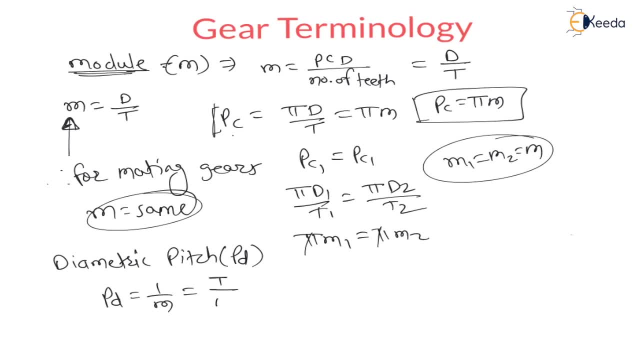 Therefore, we can say: is equal to Number of teeth divided by Pitch circle diameter. This is diametric pitch, which is reciprocal of module. Right And my dear students, Same like module, Diametric pitch is also not a dimension. Module is not any dimension. 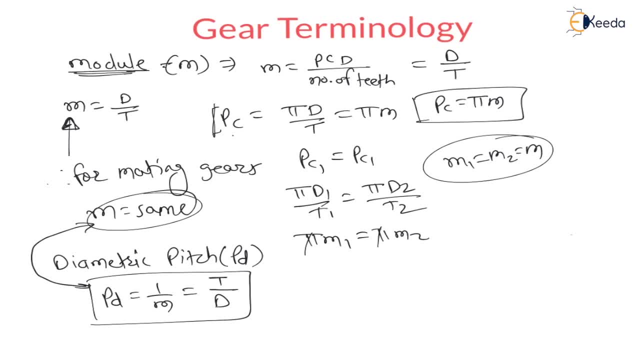 Diametric pitch is not any dimension Right Now. what is the unit of module? What is the unit of module? Module is nothing but Pitch circle diameter divided by number of teeth. Therefore M, M And unit of diametric pitch is.